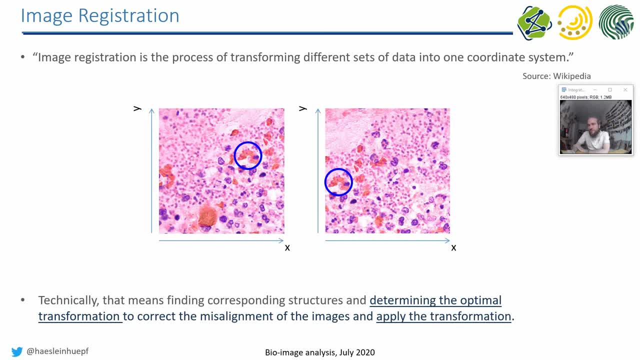 and, second of all, applying this transformation, And this is also often called image fusion. So you see here in this image, so you see here in these two images, there is the same structure in both images, And so we can likely take this corresponding structure, which is imaged twice in. 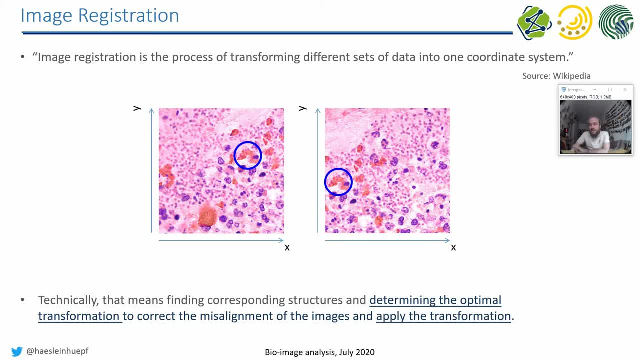 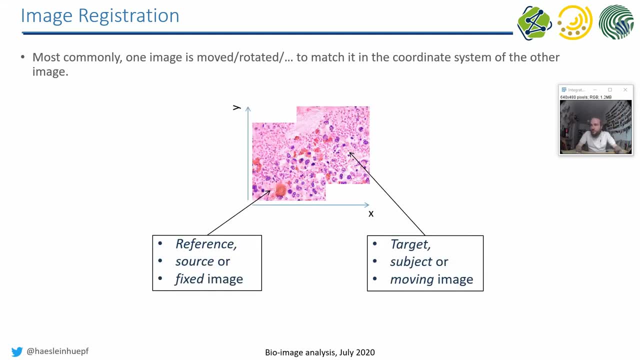 these two tiles in order to figure out a transformation which brings these two images together in one coordinate system. This is what image registration is doing, And depending on which software you work or who you talk to, you will realize that there are different terms for actually the same thing. So usually we transform one image. 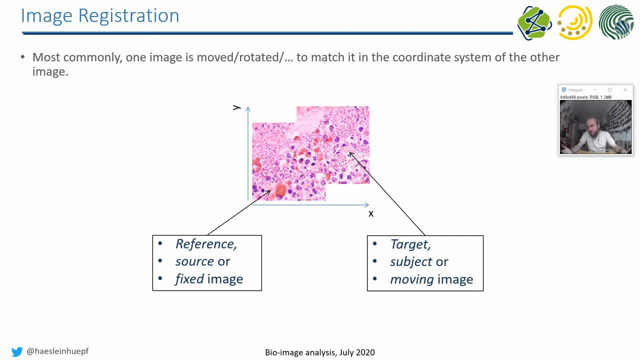 from one coordinate system into another coordinate system, the coordinate system of another image. so we basically have one fixed image. that's why it's called like that- or the reference image, or the source image, something like this- and we try to bring the other image into the same coordinate. 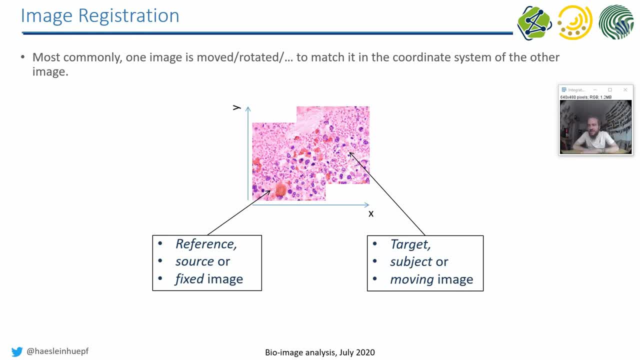 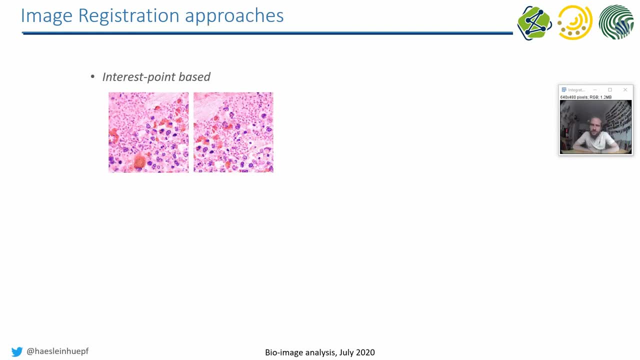 system, which is the target image or the moving image. so, in terms like that, you find them in softwares which do this and, furthermore, there are different approaches of how to do this. so, for example, one of the most, let's say, efficient ways of doing it is finding corresponding points and structures. 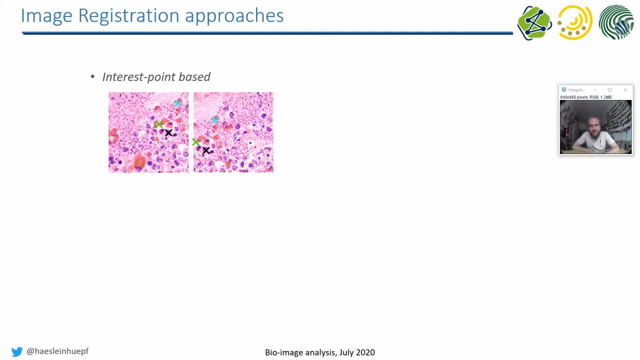 interest points in these different images, like you see here with the crosses, and then filling a system of linear equations with the coordinates and finding the perfect or the optimal solution for bringing these two images together in one coordinate system. and there's a potential alternative. so algorithms also exist, intensity based, and they basically take the two images. 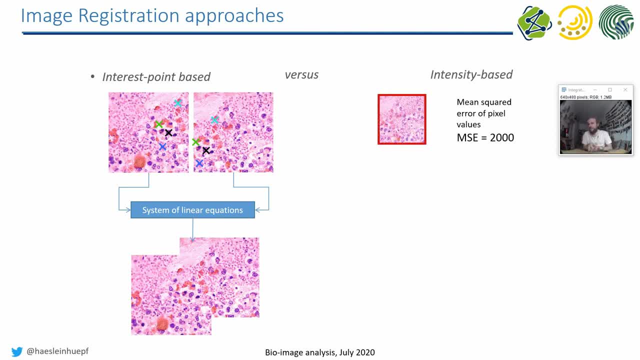 overlap them as they are and compute kind of an error between them, for example the mean squared error, and then they move this image in a certain way, and then they move this image in a certain way, and then they move this image in a certain way bit, and they do this in the image parameter introduced to you last week and 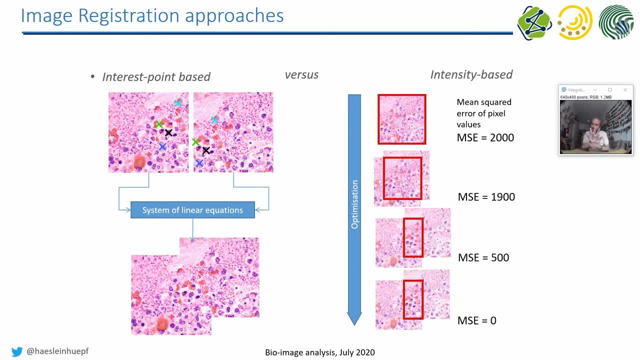 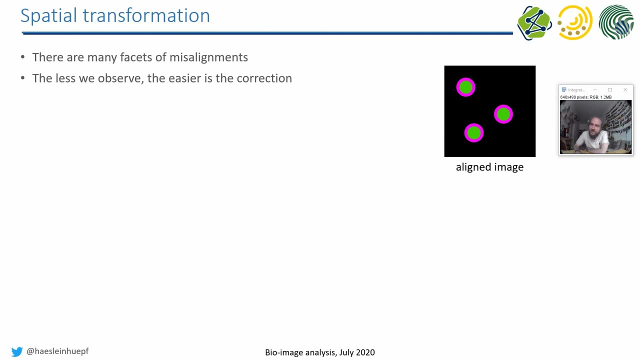 then you, by doing this a couple of times and finding the best way towards a global optimum, allows you at some point to reduce the mean square error between these two images, which allows you to find the right transformation to bring these images together. and there is different this different ways of. 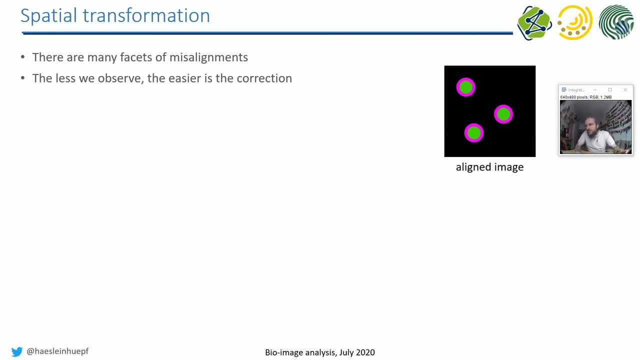 misaligning images. so let's assume we have a two channel image. we have some nuclei over here and around the nuclei there's some nuclear envelope and the image, these two with two different fluorescent markers. so we have in magenta and green these two structures and two channels in an image, in a theoretical image, if these two 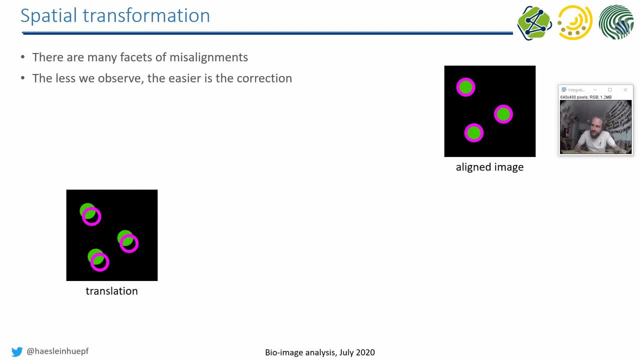 channels are translated to each other. it may look like this, and you can then apply an algorithm which finds the perfect translation vector in order to correct for this. furthermore, they can be rotated. furthermore, they can be isometrically scaled, so that means in all direction there is a factor applied making these things. 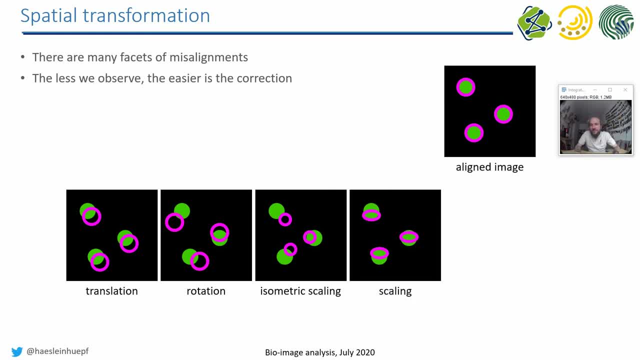 smaller or larger, so the images are scaled. but scaling can also mean that the factor is different in different directions, which makes it of course more complicated to figure out the right transformation for correcting this, last but not least, shearing. so that basically means that you have kind of such, a such 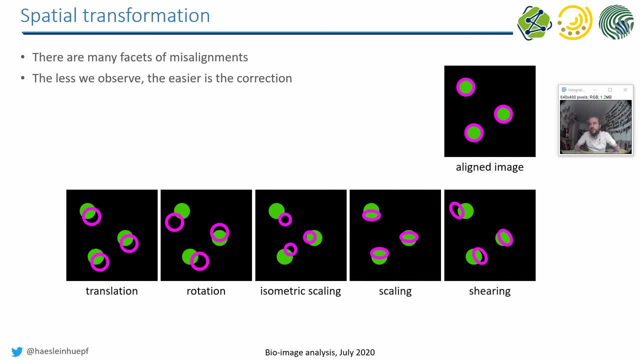 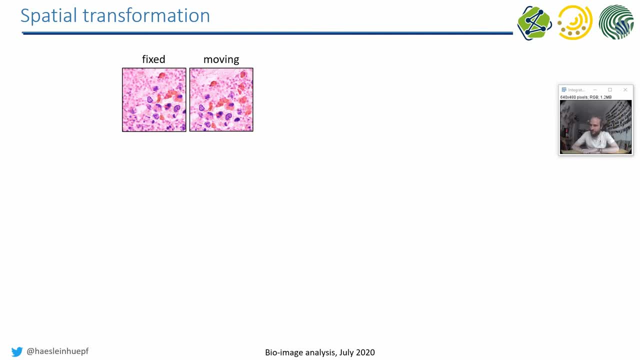 a movement within your image. shearing the image apart or one of the images apart and correcting for this might be even more complicated. and when you bring these different ways of misaligning images together, you you have another, some more terms describing the combinations of these misalignments. so let's assume the one image is just moved. 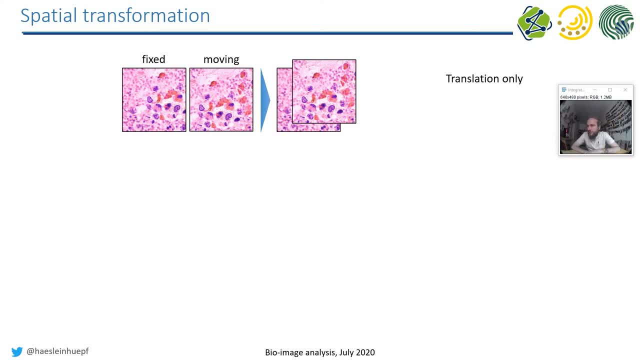 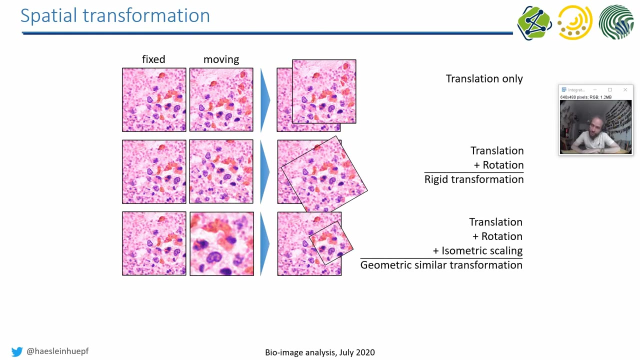 it's just translated to the other that we are talking about a translation or translation registration, which has to be applied afterwards if a translation may be present and a rotation, then we are talking about a so-called rigid transformation. if we find or if we realize that the image is translated, rotated and 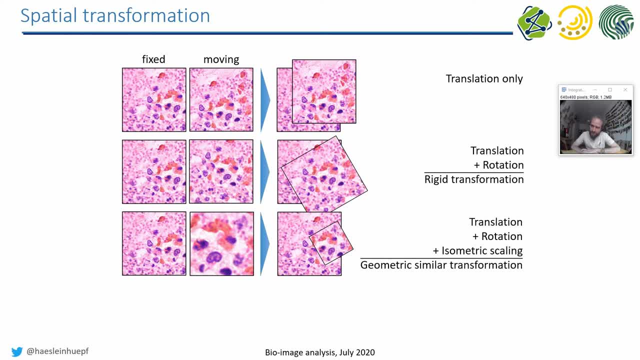 isometrically scaled. then we find terms like the geometry geometry, geometric similar transformation or some some. some software also calls it the geometry transform- I'm not sure if this term is correct, but you find these and if you have also the non-isometric scaling and shearing there, and then we are talking. 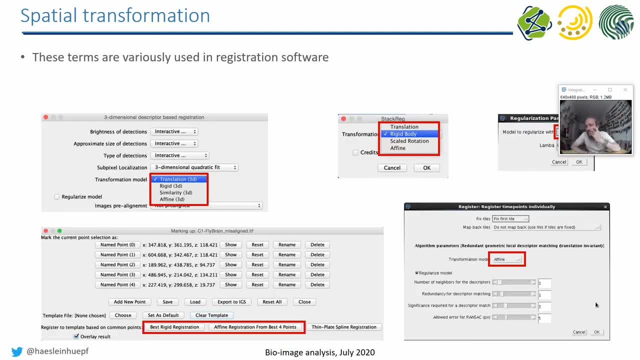 about the so-called defined transform. so why am I telling you this? because, depending on with which software you work, you find in these different pull downs, for example, you find the selection of the of the transformation you would like to correct. and a general hint is always, if you have 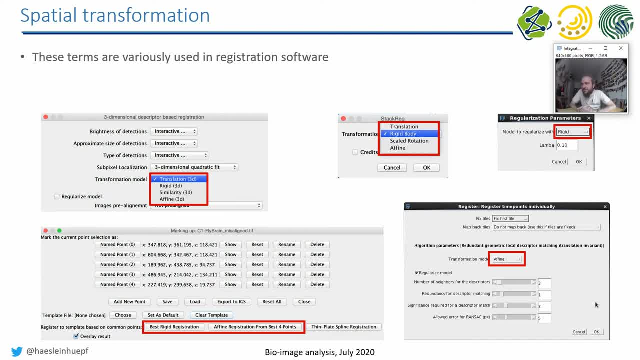 if you observe and misaligned language is just the translation, then try to correct for that with just a translation. don't use the affine transform, even though the affine transform also contains the translation. the idea is a bit: give the software the minimum possibility to do something wrong to get the best result and also to 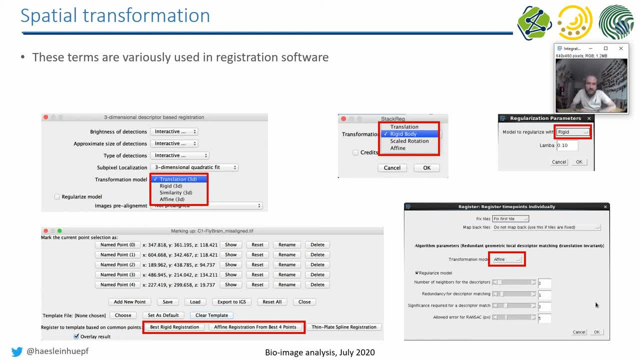 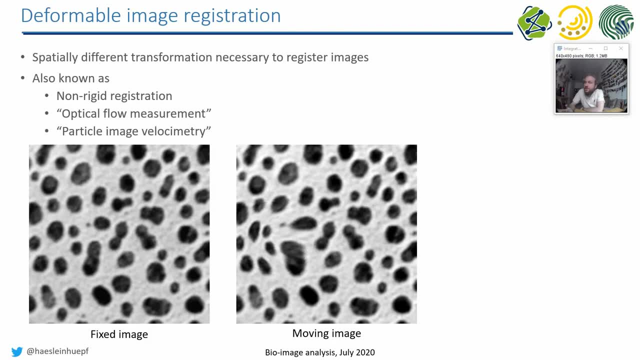 get the result in the fastest way out. so it's basically a hint when using software like that. furthermore, on top of this- so so far, we are always talking about applying a transformation to the whole image, so basically all the pixels are transformed in the same way. there is also a transformation, which is then the 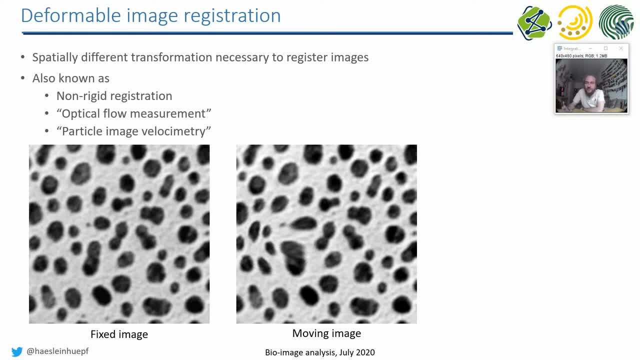 so-called non rigid transform or a performable image transformation, which can also be present as in microscopy. really observed it sometimes and maybe you see it here in the bottom image. there is obviously in this region. in these two images there is a local misalignment, so the misalignment transformation of pixels may be. 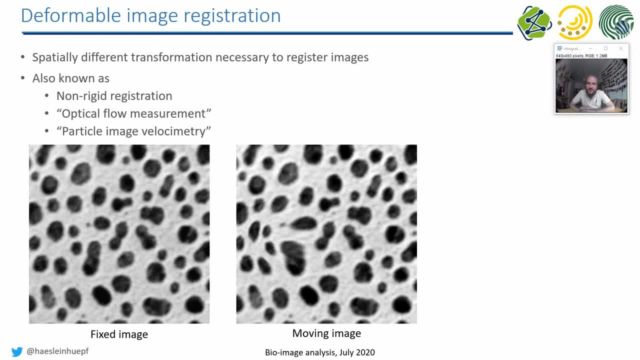 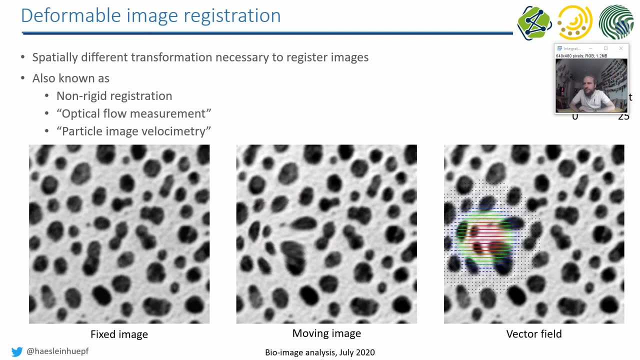 different depending on regions in the image, and that's then we are talking about deformable image registration, or sometimes also to refer to as particular image with loss, symmetry or optical flow measurement, and these transformations are typically quantified or visualized with vector fields. so you see here in this image colored lines and the 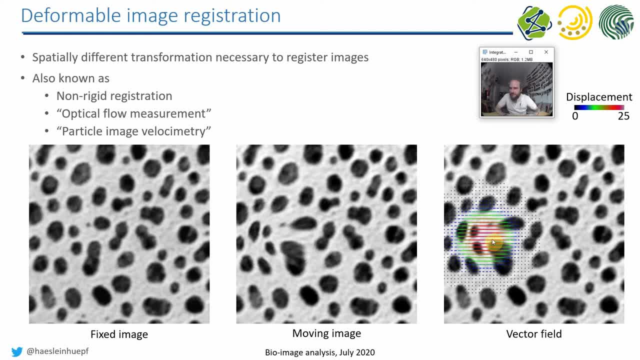 color here, in this case, represents the displacement in pixels. so here, at the very center of this region, pixels are transformed to the left or to the right, in this case, in this region, by 25 pixels, and the more you go away from that region, this displacement goes down and becomes zero, some, somewhere outside, but 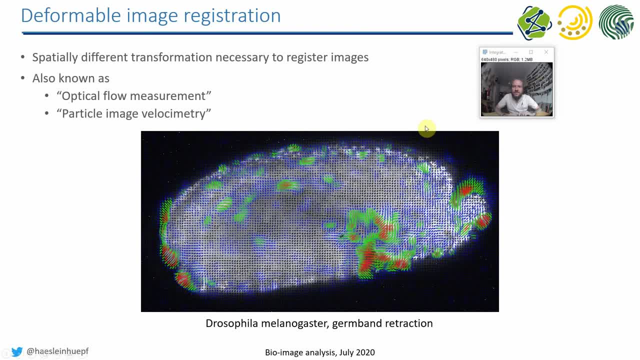 you may want to. okay, what? what do we do with that? it allows us, for example, in video sequence, it allows us to measure the flow of objects or the the motion of cells, in a general image perspective point of view. so we are not tracking objects here, so we are not following. 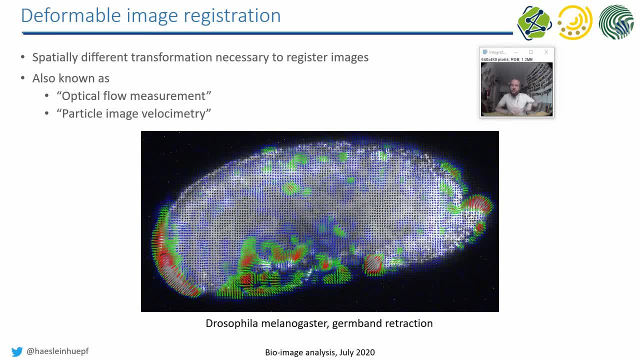 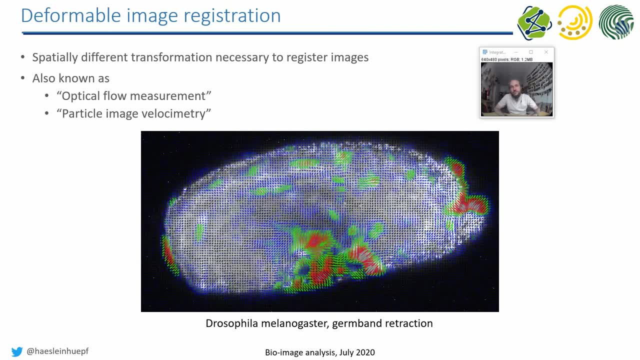 individual nuclei, even though we could right, we are following the whole structure pixel by pixel, basically, and summarize that in a visualization vector field. so this is what in microscopy most people talk about: optical flow measurement or particle image with loss symmetry. in medical imaging, usually people call it. 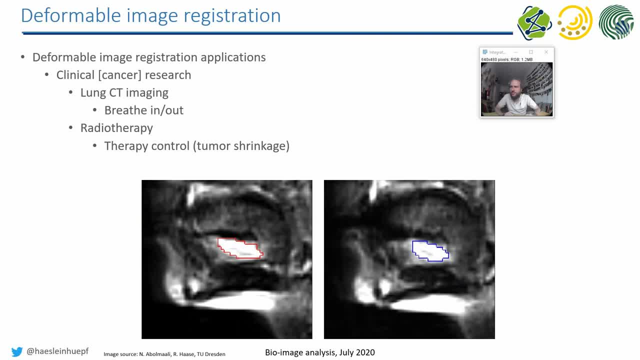 deformable image registration and here you see an example from the from. from a clinical perspective. so this is an MRI data set and I outlined here a region that's the base of the tongue. so it's so, it's not so. the patient was actually a colleague of mine, imaged in the MRI and we outlined the base of the tongue and we 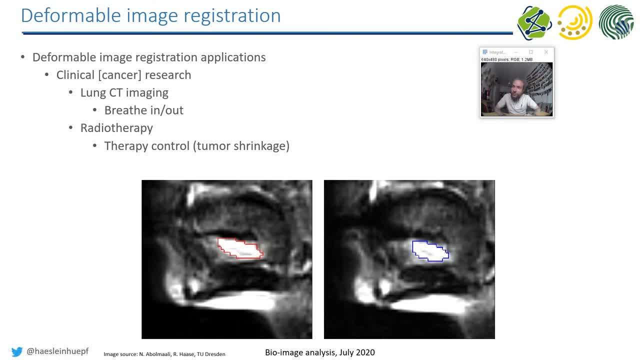 asked the patient, the volunteer, to open her mouth, and then the tongue is basically falling to the back. so we wanted to to measure the misalignment of these two roi's, which is obviously a local thing, which is obviously not a global transformation of the whole image, because only the tongue 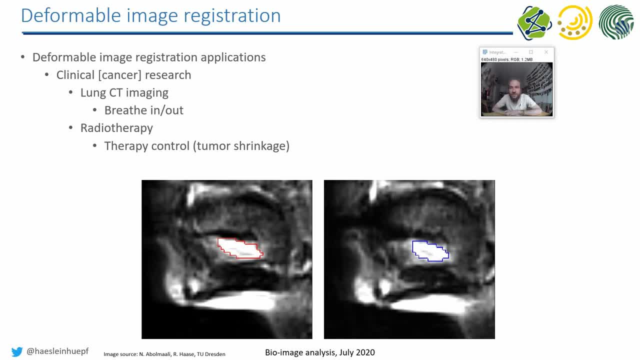 and the mouth are moving- and this is quite relevant when you think about radiotherapy and the tumor, for example, in this region- then if you want to hit this tumor coinciding, then you have to, you have to take these kind of transformations into account in order to make an ‎eye and an outline, so to speak˚. 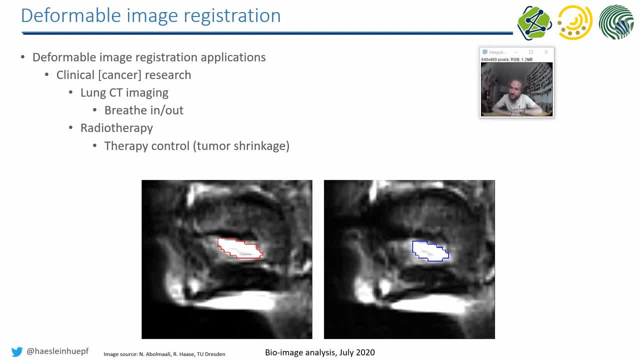 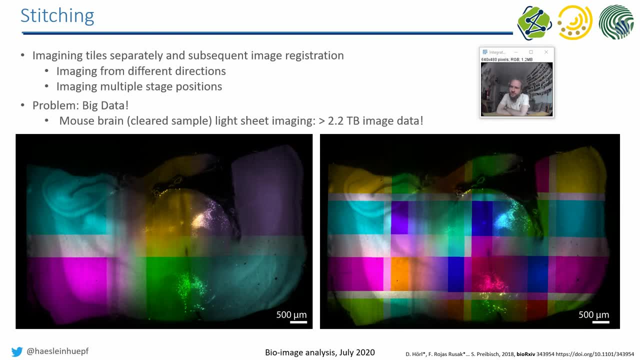 of an anatomical structure precise, or to figure out how precise we can do these things. But what is the term you often find in microscopy, More and more actually in recent years, is stitching. So when the structure we are looking at, so we're looking at here. 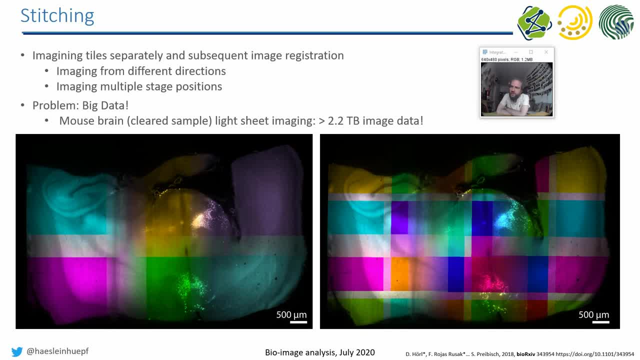 we are looking at the mouse brain, when the structure we are imaging is too big for our microscope, so the field of view of the microscope is not large enough to capture the whole scene, the whole sample. then we have to take several images, tiles, and then stitch these tiles. 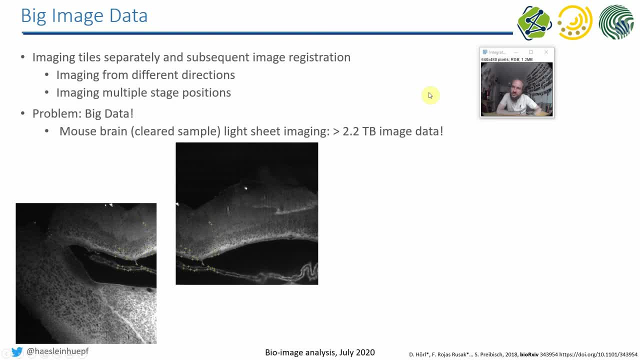 together. afterwards, Especially when this image data becomes very big, it becomes a problem. I was talking a bit about tiling and big data last week, So when you look here, for example, this is again also a mouse brain, same image as before, and you see here that with 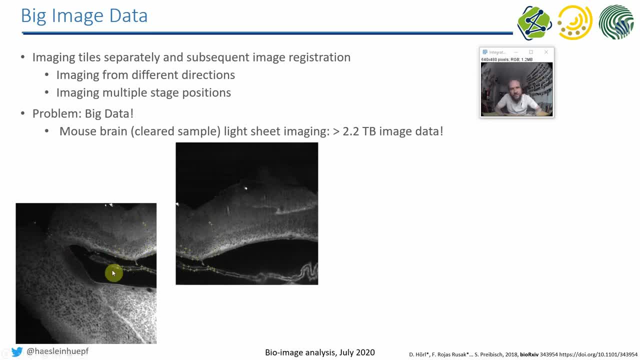 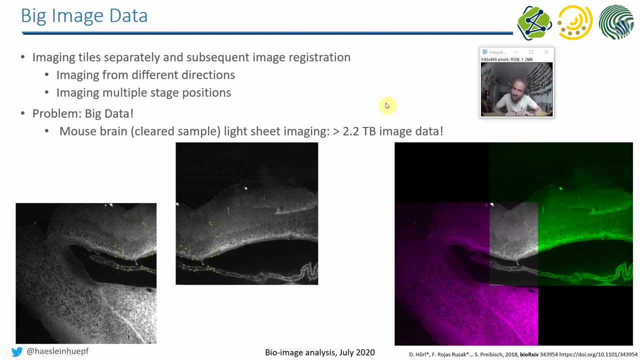 typical ImageJ functionality. the developers were here showing some interest points And the challenge is now to bring these interest points together so that this over to these two sections taken from the mouse brain image from the mouse brain and fit together in one data set. But technically this is feasible today. 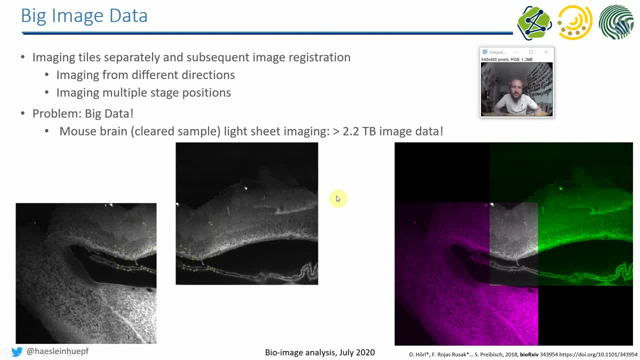 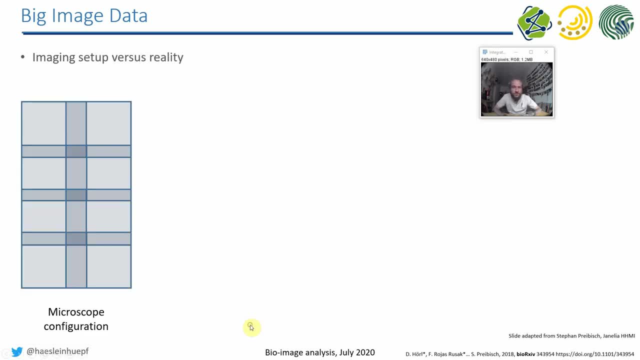 I will show you a tool that you can use for that. I'm just saying that for big data. it's a bit challenging if you work with terabytes of image data. So why is it challenging? Imagine you have a structure elongated a bit in this direction. 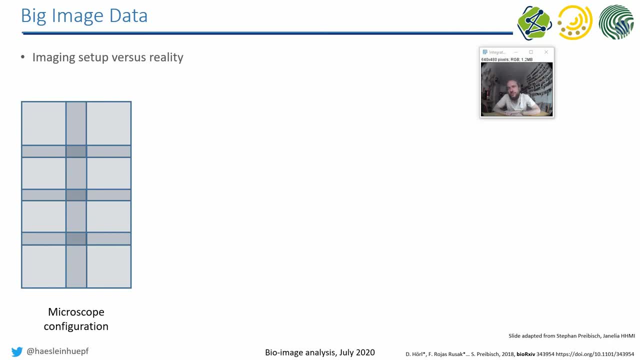 and you would like to image it. you realize it does not fit in the field of view. So you realize that you have to take eight fields of views and have to image them. So this is how you basically set up your microscope, And then you click on run And when you are done with imaging you realize that the microscope was 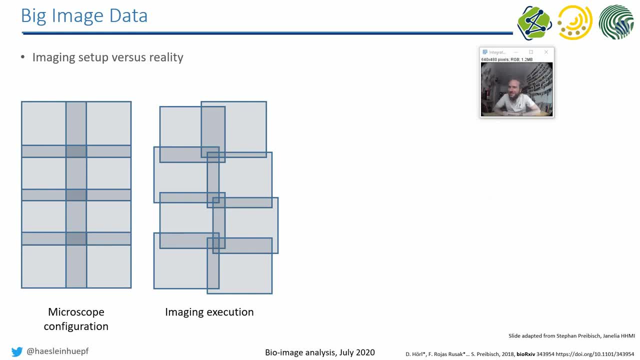 to some degree doing what it was supposed to do, but not precisely, And there are many reasons for that. So it's not just the microscope stage does not move, as you would like to, It also has something to do that when light propagates through thick tissues it is some. 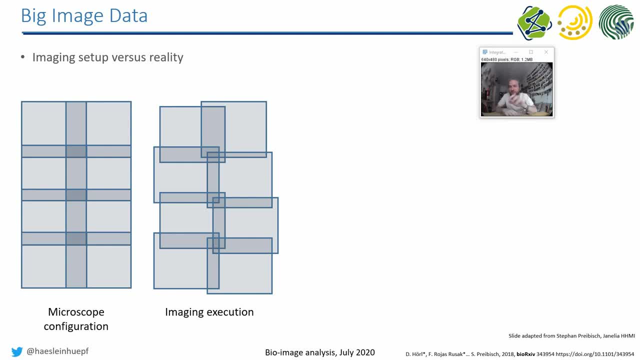 sometimes not going straight, because refractive index differences make the light a bit propagate in nonlinear ways And then afterwards what you get in your images may look like that. So you actually have acquired tiles from these positions and not from the positions as you. 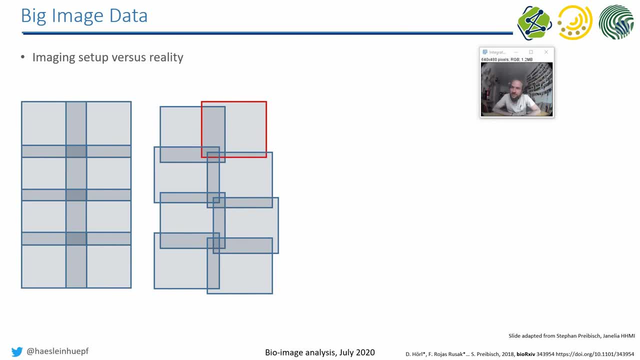 configured it And each of these tiles is half of your computer memory, or let's say a quarter of your computer memory. So you cannot put all eight tiles in the computer and register them And stitch them, And you have to do this basically starting from one tile of interest at the moment. 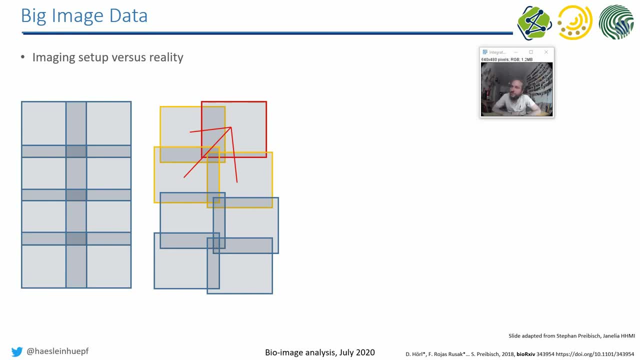 to the neighbor tiles and maybe tile by tile And from each tile to each neighboring tile, and always do this pairwise. And when you can do this pairwise and you can do this from different tiles, you don't have to have the whole data set with all eight tiles or with all 1000 tiles. 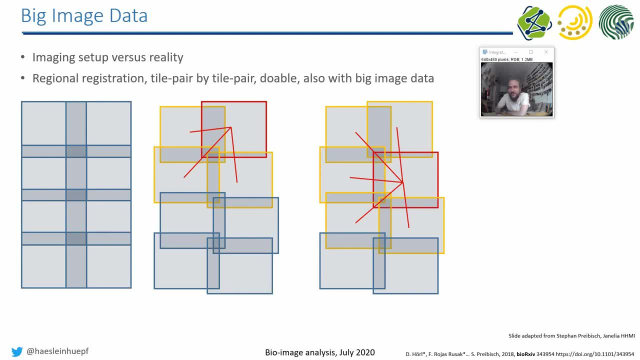 in computer memory. You only have pairs or have to have pairs of them, And this is actually the thing which makes the big image data stitching possible. At the end, you take all these transformations which have been determined between these different tiles and you still have to equalize a bit the error between them in order to figure out how all these 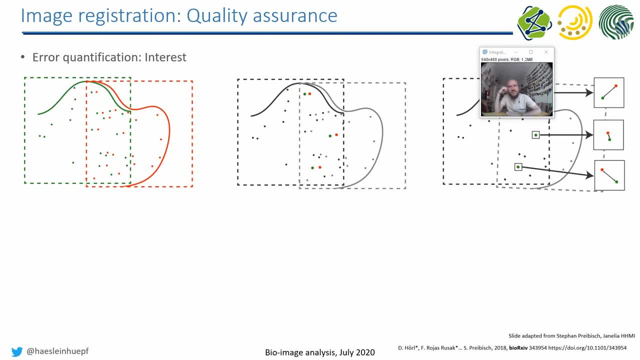 tiles fit together in the very best way. And then, when you have aligned all your tiles, then you should still do some error quantifying. So you see here, for example, how these overlapping tiles and the interest points in them are then taken to measure, for example, an average distance between the interest points of